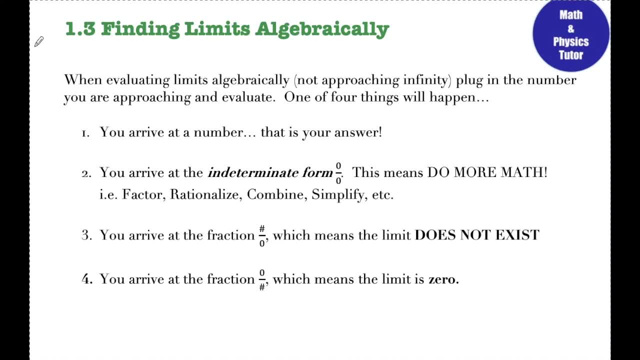 Hi everyone. today we're going to be talking about finding limits algebraically. So when I evaluate a limit algebraically, I'm always first going to plug the number that I'm approaching for my limit in for whatever variable I'm looking at, and just solve and see what I get. When I do that, 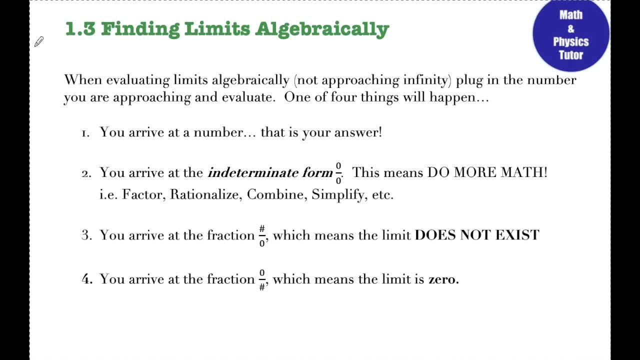 one of four things will happen that will determine if I need to do any more work or what my answer is. So the first thing that happens is I plug in my numbers and I get an answer. Perfect, I get a number over a number. There's my answer. I'm good to go. The second thing that can happen is once 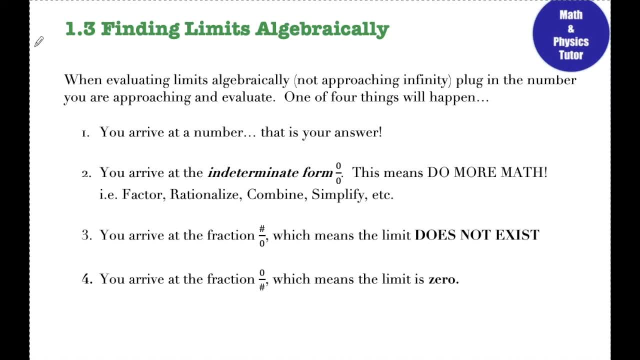 I've plugged in my numbers and evaluated, I end up with zero over zero. This is an indeterminate form and means that I need to do more math. That means that I need to either factor, rationalize, combine, simplify etc. Something to change what that expression looks like and then re-evaluate. 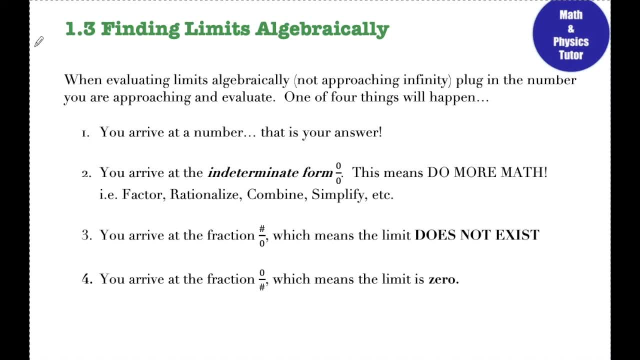 that limit again. The third thing that can happen is, once I've plugged in my numbers, I end up with a number over zero, Five over zero, Eight over zero, Whatever Something, number over zero. This means that the limit does not exist. That's a DNE limit. The fourth thing that can happen: once 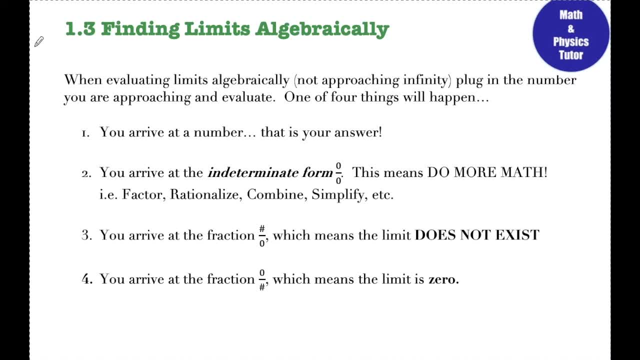 I've plugged in my numbers is I end up with zero over a number, Zero over one, Zero over five, Zero over negative 20.. That means that my limit is just zero and I don't have to do any more work. Let's look at a couple of examples with each of those scenarios. Number one: the limit as x. 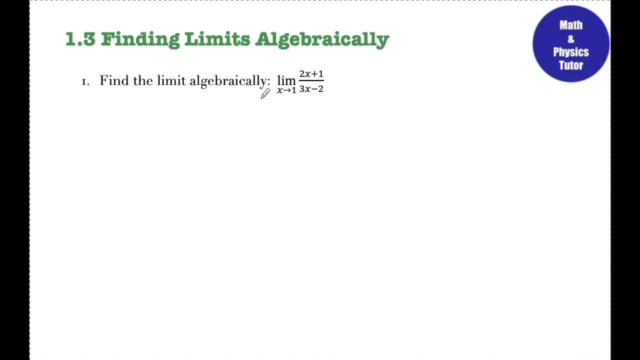 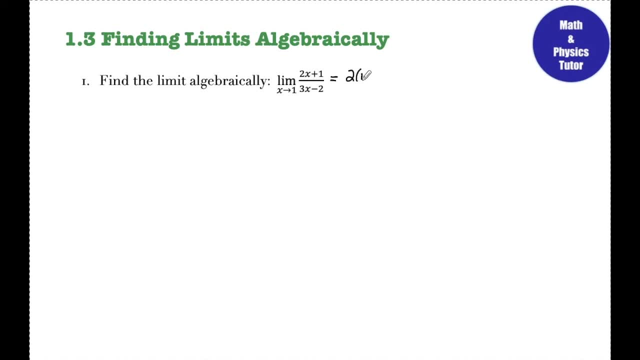 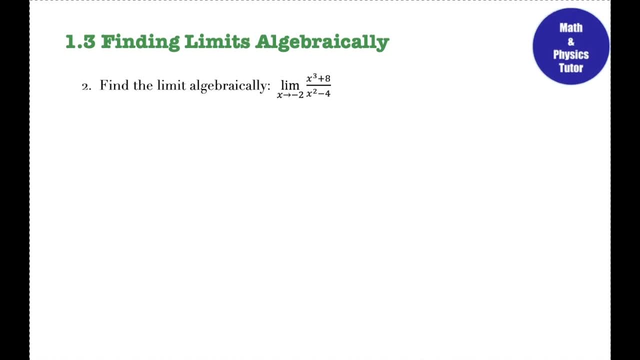 just three, No need to do any more work. Number two: the limit as x approaches negative two of x cubed plus eight over x squared minus four. So again, the first thing that I'm going to do is plug negative two in for x. So I have negative two cubed plus eight. 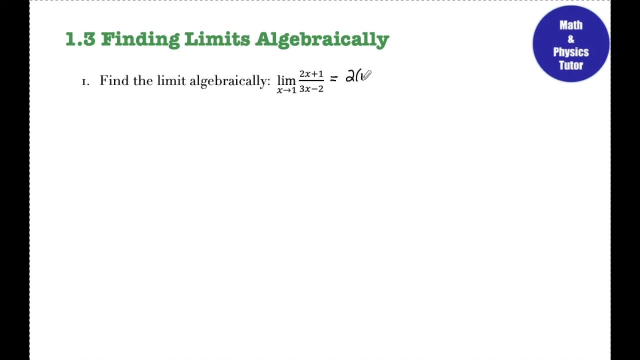 to plug in my number that I'm approaching in for the variable. So I'm going to have two times one plus one over three times one minus two And I'm just going to evaluate here. So in my numerator I get three, In the denominator I get one. So my answer here is just three. No need to do any more. 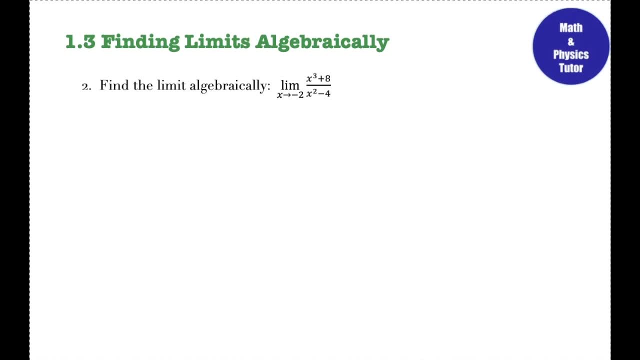 work. Number two: the limit as x approaches negative two of x, cubed plus eight over x, squared minus four. So again, the first thing that I'm going to do is plug negative two in for x. So I have negative two cubed plus eight over x, squared minus four. So I'm going to plug in my number, So I 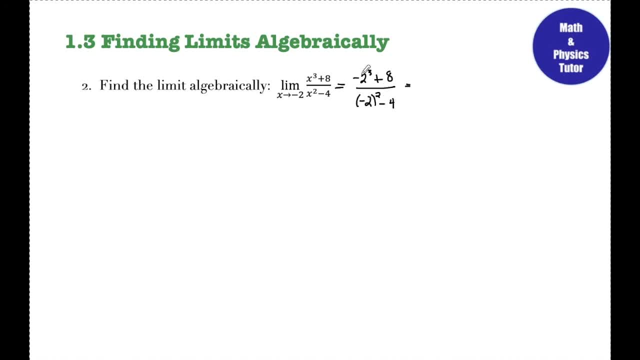 over negative. two squared minus four. In the numerator this is gonna be negative eight plus eight, so that's zero. And in the denominator I'm gonna have four minus four, so that's also zero. So this is the case where I have an indeterminate form. 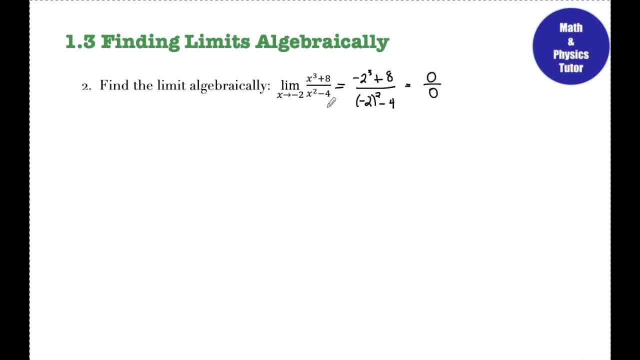 I have to do more math, I have to do something to this expression to get things to cancel out and then try plugging in that negative two again. So I'm first gonna just rewrite the problem, And when I look at this expression I can see that the numerator is a sum of cubes. 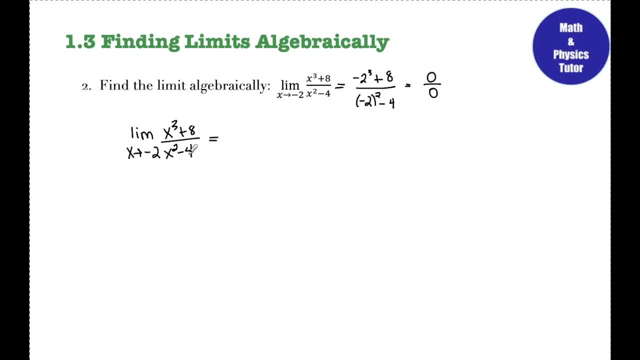 so I can factor that. And the denominator is a difference of two squared, so I can factor that as well When I rewrite this expression. before I start simplifying, it's very important that you keep rewriting your limit piece in the beginning. You can't just drop the limit piece. 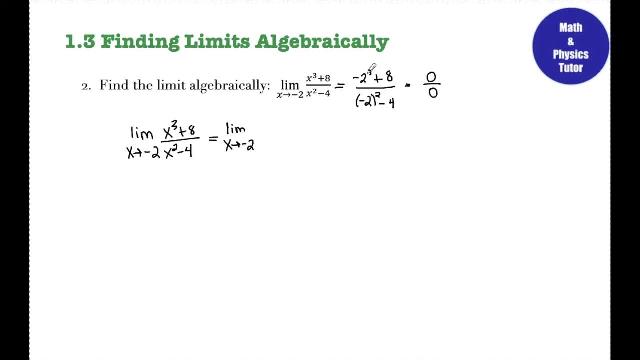 and rewrite the expression. You have to keep rewriting the limit piece until you plug in numbers. That's why I was allowed to drop the limit here. but I'm not going to drop the limit just yet here In the numerator when I factor a sum of cubes. 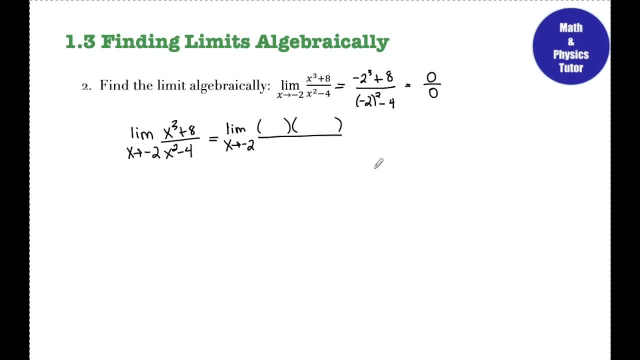 I set up a small set of parentheses and a bigger set of parentheses. I know the signs in the parentheses are same opposite positive as what was already in the numerator. So I'm gonna have same opposite positive. Now I just have to figure out the terms. 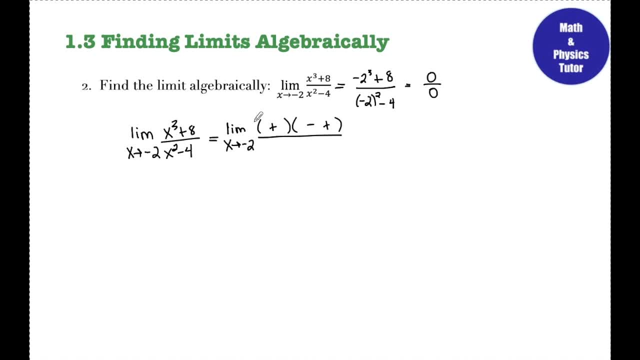 that go in each of these. This first term is always the cube root of the first term, so that's x. This second term is always the cube root of the second term, so that's two, The first term in that bigger set of parentheses. 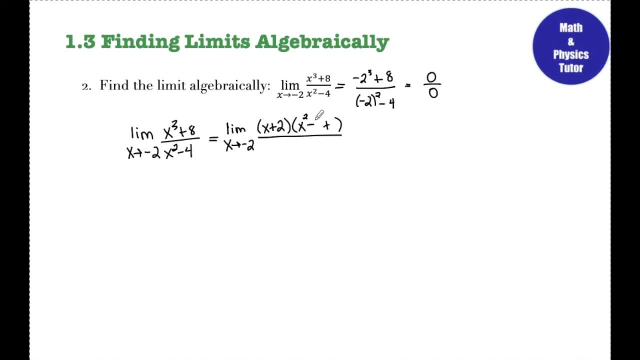 is this term squared. This middle term is a combination of these two terms, so two- x, And that last term is this second term squared, so four. In the denominator I have a difference of two squares, so I know that's just x plus two and x minus two. 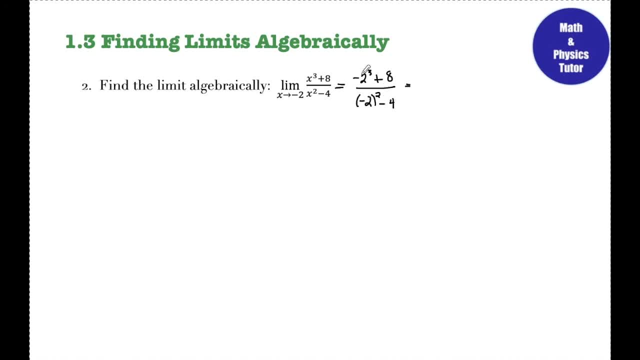 over negative 2 squared minus 4.. In the numerator this is going to be negative 8 plus 8, so that's 0, and in the denominator I'm going to have 4 minus 4, so that's also 0.. So this is the case where I 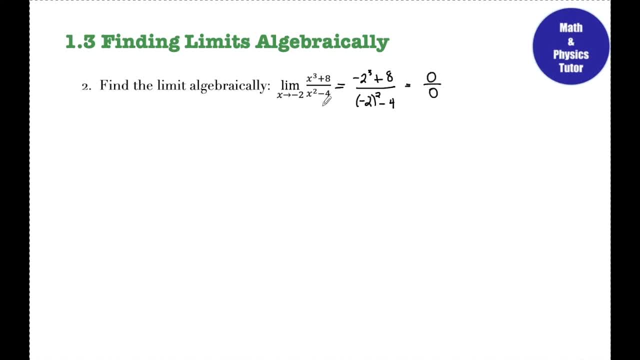 have an indeterminate form. I have to do more math, I have to do something to this expression to get things to cancel out and then try plugging in that negative 2 again. So I'm first going to just rewrite the problem and when I look at this expression I can see that the numerator is a sum. 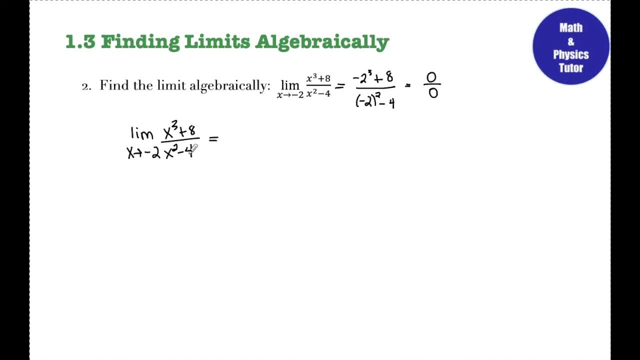 of cubes, so I can factor that. and the denominator is a difference of 2 squared, so I can factor that as well When I rewrite this expression. before I start simplifying, it's very important that you keep rewriting your limit piece in the beginning. You can't just drop the limit piece and rewrite. 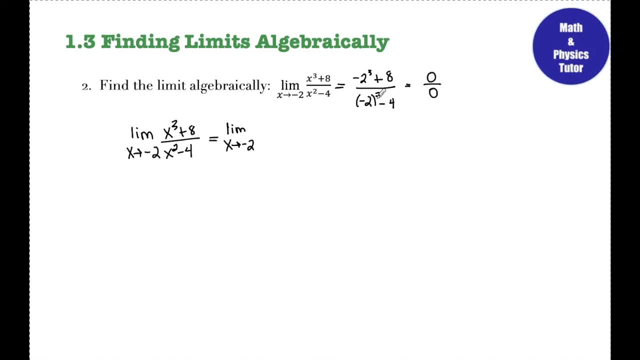 the expression. You have to keep rewriting the limit piece until you plug in numbers. That's why I was allowed to drop the limit here, but I'm not going to drop the limit just yet here. In the numerator, when I factor a sum of cubes, I set up a small set of parentheses and a 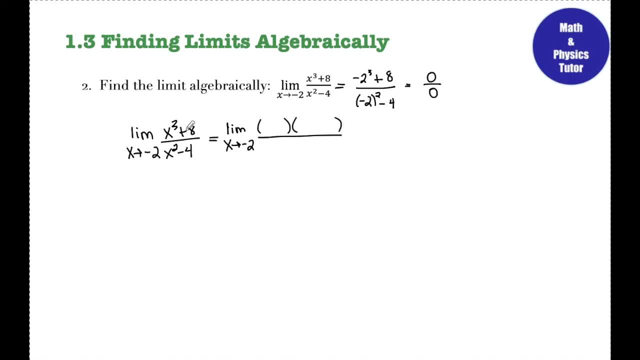 big sum of cubes, I set up a small set of parentheses. and a big sum of cubes: I set up a bigger set of parentheses. I know the signs in the parentheses are same opposite positive, as what was already in the numerator. so I'm going to have same opposite positive Now I just have to. 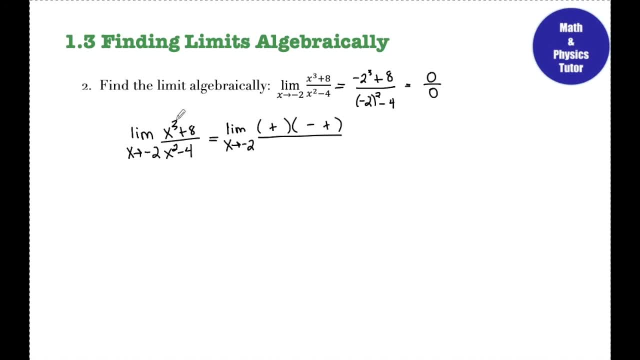 figure out the terms that go in each of these. This first term is always the cube root of the first term, so that's x. This second term is always the cube root of the second term, so that's 2.. The first term in that bigger set of parentheses is this term squared. This middle term is a. 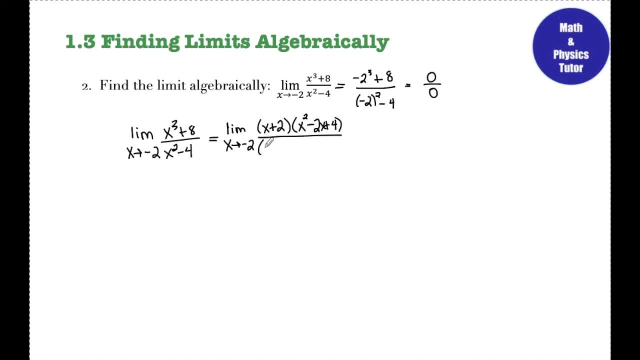 second term squared, so 4.. In the denominator I have a difference of two squares. so I know that's just x plus 2 and x minus 2, and now I can see that my x plus 2 in the numerator cancels with the x plus 2 in the denominator. So now I can evaluate the limit as x approaches negative 2. 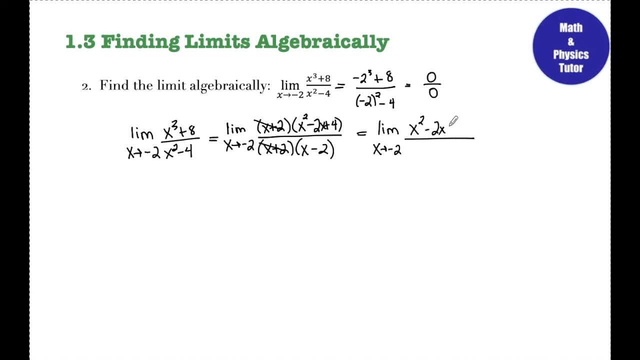 of what I have left over. So x squared minus 2x plus 4 over x minus 2.. Now I'm going to plug the negative 2 in for x and since I'm doing that, I can drop that limit in the front. So negative 2 squared. 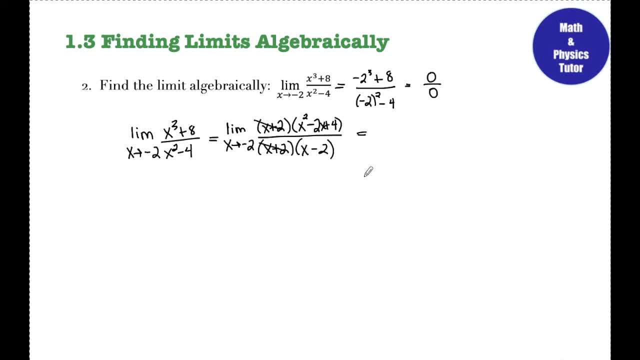 And now I can see that my x plus two in the numerator cancels with the x plus two in the denominator. So now I can evaluate the limit as x approaches negative two of what I have left over. So x squared minus two, x plus four over x minus two. 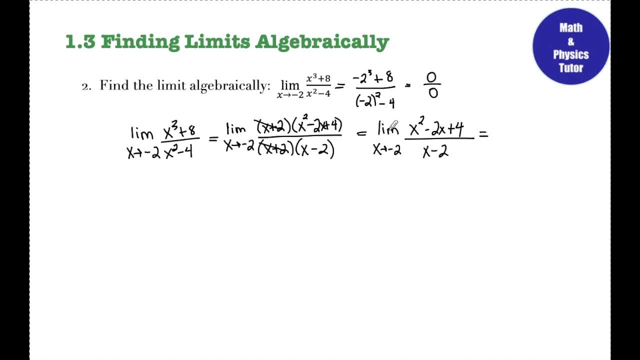 Now I'm gonna plug the negative two in for x, and since I'm doing that I can drop that limit in the front. So negative two squared is four. two times negative two is positive four. Bring that plus four over, And then in the denominator I have negative two minus two. 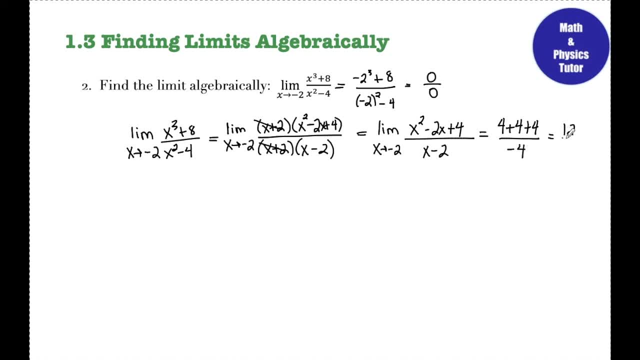 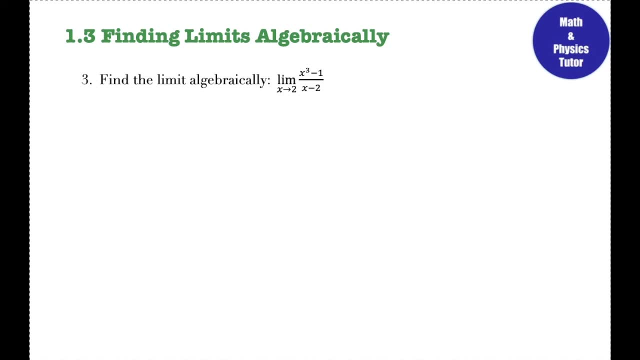 so that's negative four. So now this becomes 12 over negative four. So my answer is negative three. Number three: the limit as x approaches two. of x cubed minus one over x minus two, I always have to plug in that number first. 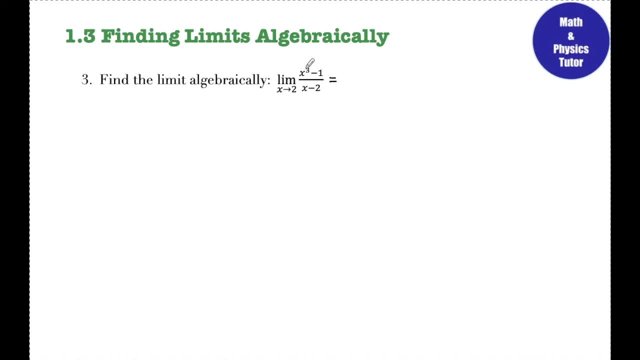 and see what's going on. So if I plug a two in two, cubed is eight minus one is seven. over two minus two is zero. This is the case where I have a number over zero, So that means my limit does not exist. 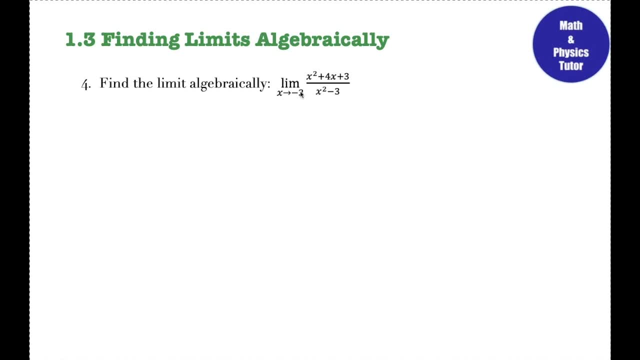 This is a DNE limit, Number four. the limit as x approaches negative three of x squared plus four, x plus three over x squared minus three. I am first going to plug in negative three for x. So negative three squared is nine. Four times negative three is negative 12.. 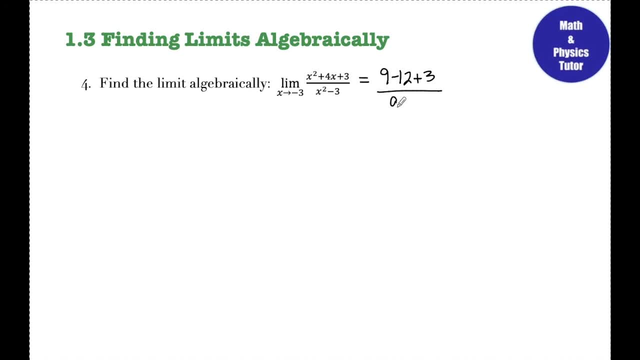 I have that plus three And in the denominator negative three squared is nine minus three. Nine minus 12 plus three is going to be negative. three Plus three is going to give me zero, And then the denominator is six. So since I have zero over a number, 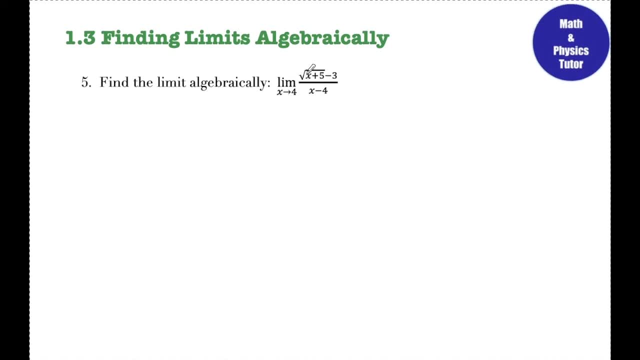 the limit here is just zero, Number five. the limit as x approaches four of the square root of x plus five minus three over x minus four. So first things first, I'm gonna plug in four for x. So I have the square root of four plus five minus three. 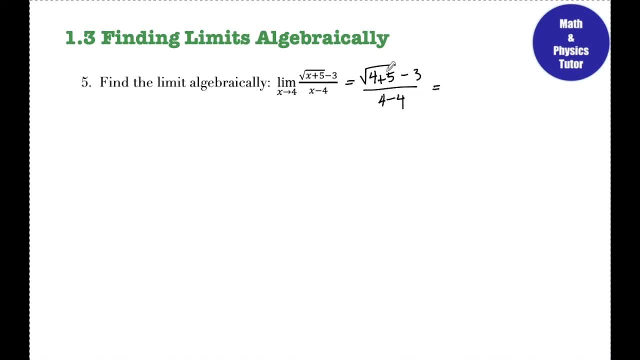 over four minus four. In the numerator four plus five is nine And I know the square root of nine is three. So my numerator is gonna be zero, Three minus three, And then denominator I also have zero. So this is that indeterminate form. 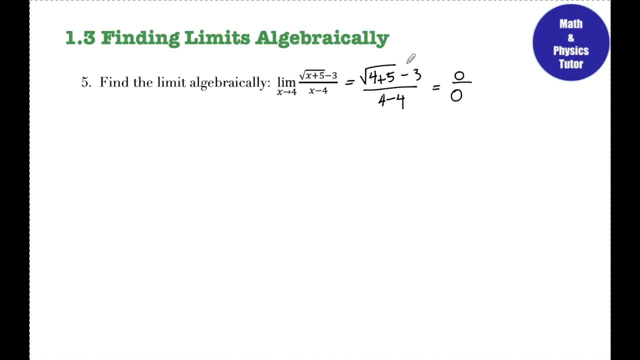 I need to do more math here. Whenever I have a radical that's giving me an indeterminate form, what I'm gonna wanna do is multiply this whole thing by the conjugate of the radical piece, So I'm gonna rewrite that original problem. 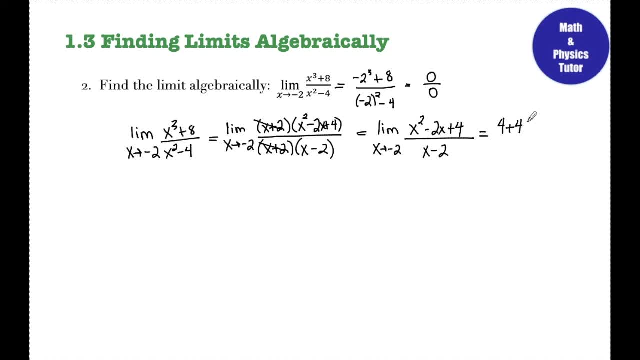 is 4.. Negative 2 times negative 2 is positive 4. Bring that plus 4 over and then in the denominator I have negative 2 minus 2, so that's negative 4.. So now this becomes 12 over negative 4. so my answer: 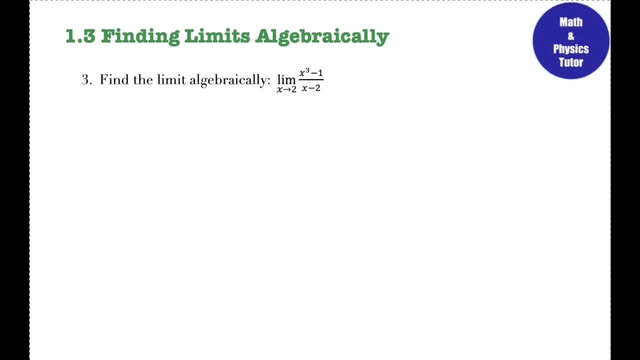 is negative. 3. Number 3. The limit as x approaches 2 of x cubed minus 1 over x minus 2.. I always have to plug in that number first and see what's going on. So if I plug a 2 in, 2 cubed is 8 minus 1 is. 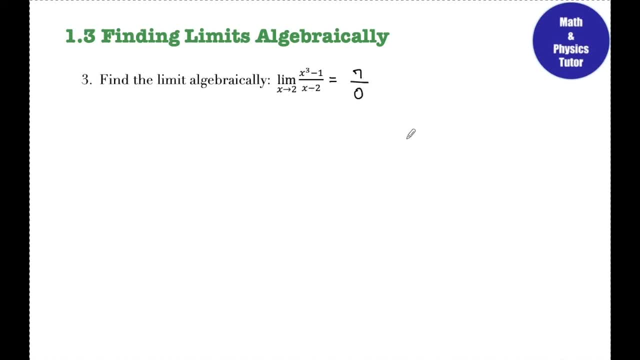 7. Number 2 minus 2 is 0. This is the case where I have a number over 0, so that means my limit does not exist. This is a dne limit, Number 4.. The limit as x approaches negative 3 of x squared plus 4x. 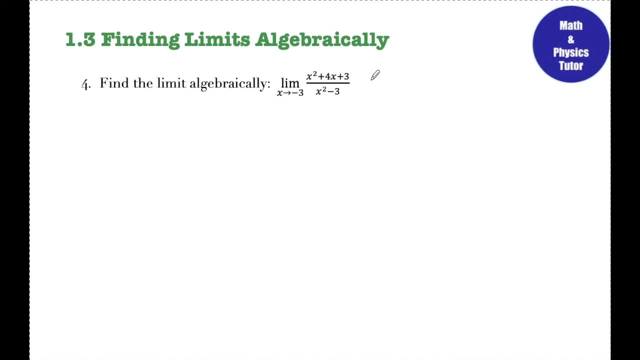 plus 3 over x squared minus 3.. I am first going to plug in negative 3 for x. So negative 3 squared is 9.. 4 times negative 3 is negative 12.. I have that plus 3 and in the denominator negative 3. 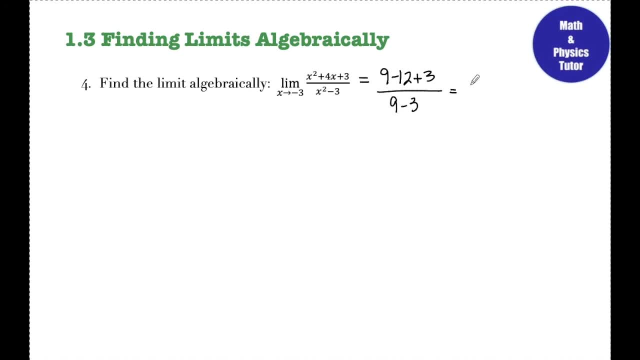 squared is 9 minus 3.. So negative 2 plus 3 is negative 3.. I have that minus 4.. So, being negative, 3 squared minus 3 plus 0.. I have 9 plus 9 is positive 3.. If it were negative 3, I would have 9 minus 48 b x here. 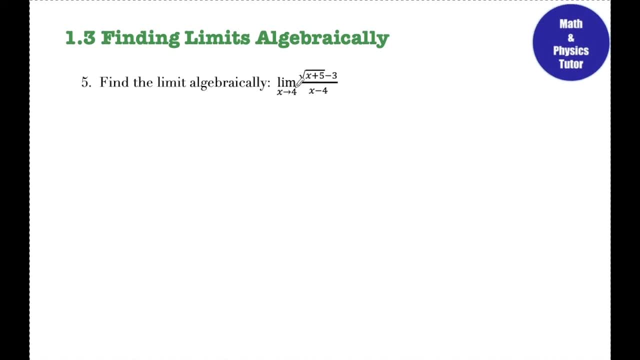 so I would have 9 number 10 minus 12 plus 9 is minus 3.. I would also be negative 3 over 4 times 4 by a factor of 2.. But if I plug in negative 3 is negative 3 over x squared plus 4 x squared. 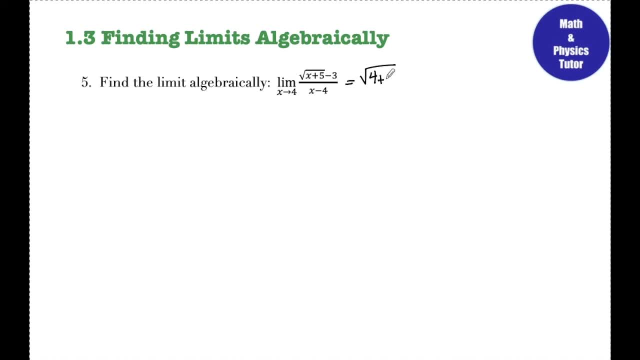 plus 3 is positive 4 and I have the denominator as positive letter 8, this part, Then I'm going to plug in negative 3 or negative 4.. What am I going to do? I'm going to plug in negative 0 over. 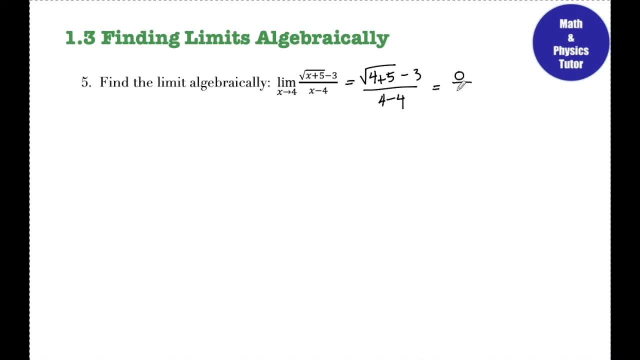 3.. So my numerator is going to be 0, 3 minus 3.. And then denominator, I also have 0. So this is that indeterminate form. I need to do more math here Whenever I have a radical that's giving me. 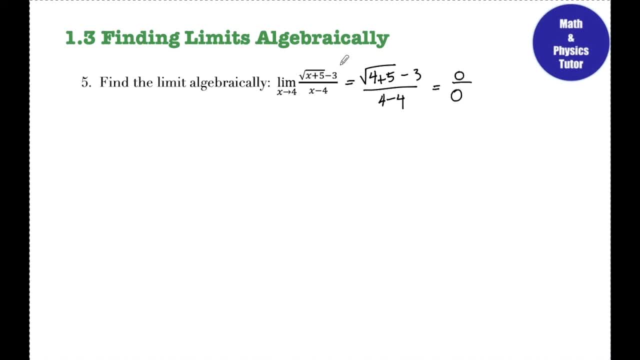 an indeterminate form. what I'm going to want to do is multiply this whole thing by the conjugate of the radical piece. So I'm going to rewrite that original problem. And I'm going to multiply the top and the bottom of this expression by the conjugate of the numerator. So I'm going to 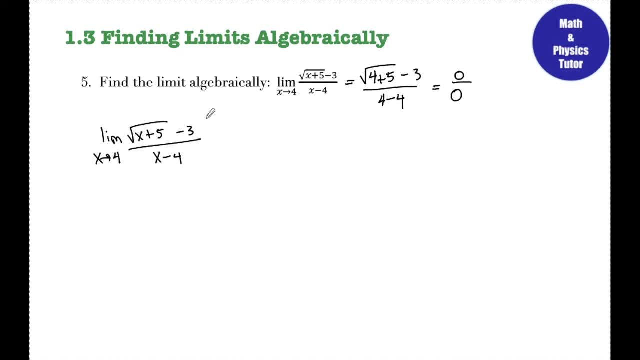 And I'm going to multiply the top and the bottom of this expression by the conjugate of the numerator. So I'm going to multiply by the square root of x plus five plus three. So to multiply in the numerator, I also need to multiply in the denominator. 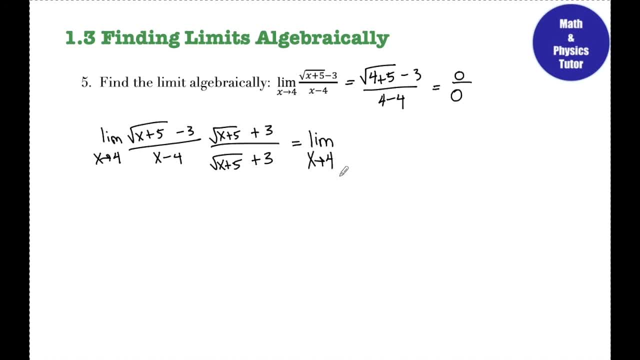 When I do this multiplication I still carry over my limit, because I'm not evaluating just yet In the numerator, I'm pretty much just foiling or just multiplying two binomials. So I have rad x plus five times rad x plus five. 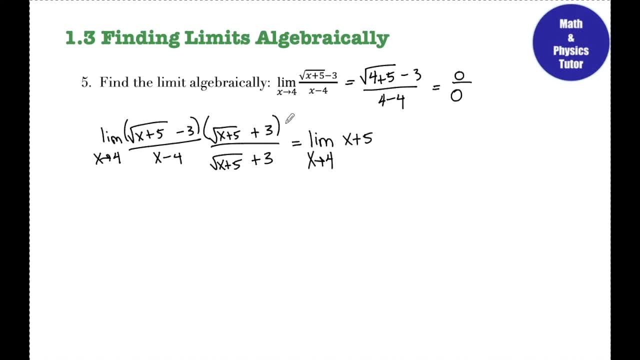 That's just gonna be x plus five. My outer two terms are gonna give me three rad x plus five, And my inner two terms are gonna give me negative three rad x plus five. So those two terms just cancel each other out other out. Next I need to multiply the negative 3 and the positive 3, so that's going to give me: 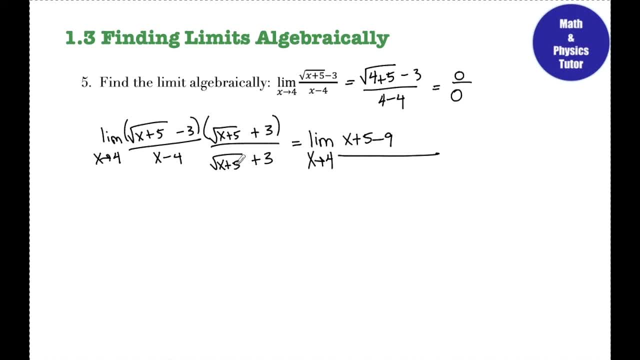 a negative 9.. So there's my numerator In the denominator. I'm not going to multiply these out, I'm going to leave this as x minus 4 in parentheses, and rad x plus 5 plus 3 in parentheses, The goal. 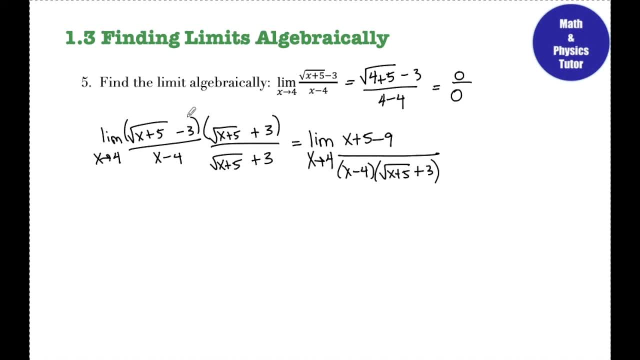 of multiplying by the conjugate in this example is to have things cancel in the numerator so it looks a little bit smaller. but now when I go to rewrite my whole expression for one more time, you'll see that something's going to cancel. So now that this is rewritten I can see that the x 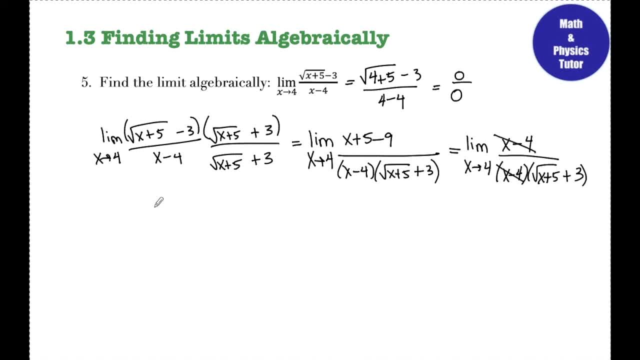 minus 4 in the numerator cancels with the x minus 4 in the denominator, leaving me with 1 over the square root of x plus 5 plus 3.. Now that this has been simplified, I'm going to plug the 4 in for x. 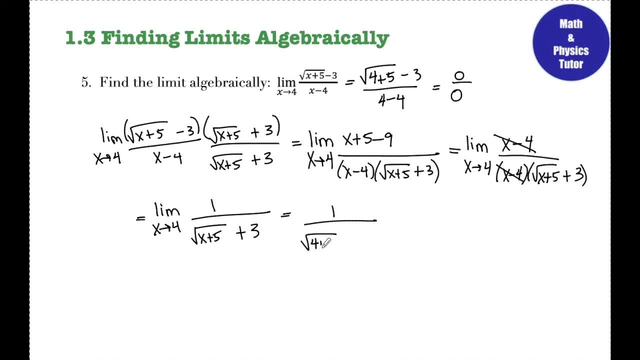 and hopefully I'm going to get an answer now. So I have the square root of 4 plus 5 plus 3 in the denominator. The square root of 4 plus 5 is the square root of 9, so that's 3, and 3 plus 3 is 6.. So the answer. 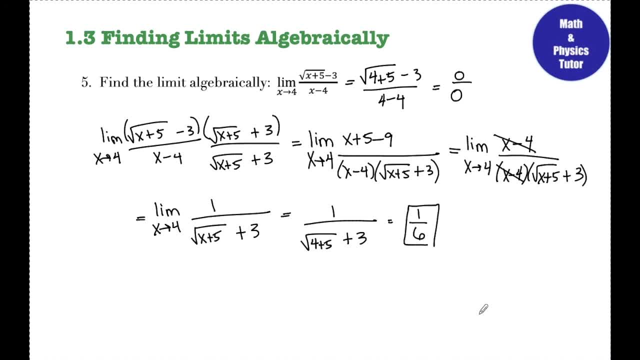 to this question is 1- sixth. That's it for finding limits algebraically. If you have any questions, feel free to leave them in the comments below, and if you'd like a copy of this worksheet- and you are not one of my students- you can send us an email and I'll leave that email in the